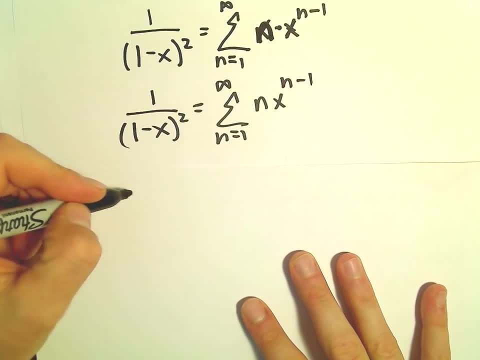 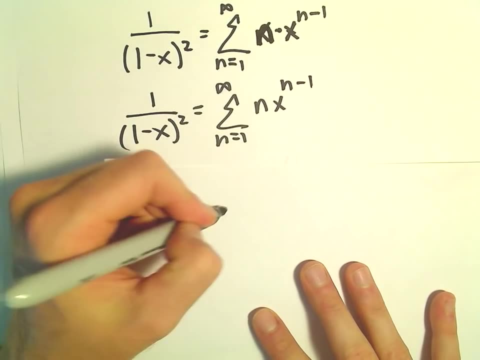 Well, I guess what we could do is we could multiply. We could multiply both sides by x, So on the left side we would have x times 1 minus x squared, And on the right side we can also multiply by x. 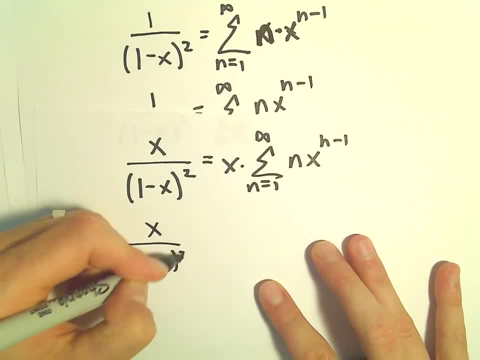 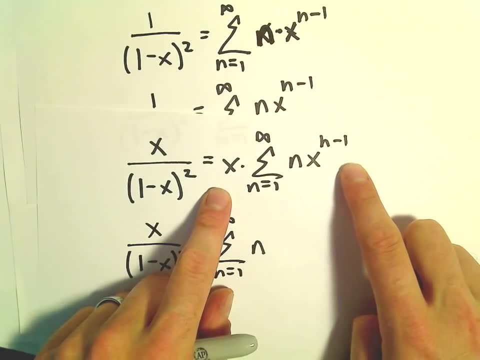 Okay, so on the left we'll have x over 1 minus x squared. On the right side we'll have the series from 1 to infinity of n, And again we can move the x inside. So since we're multiplying like bases, 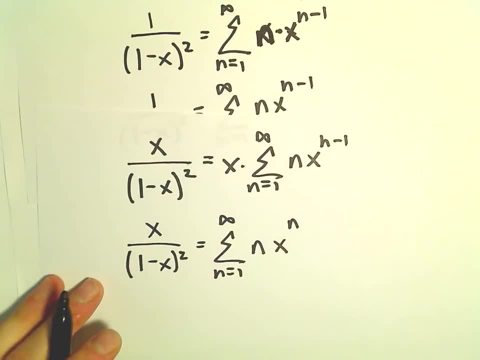 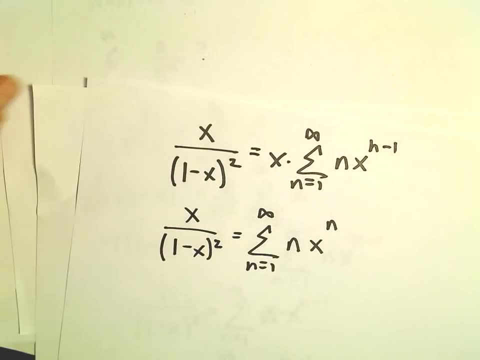 we'll be left with x raised to the n. So we'll be left with x raised to the n. So we'll be left with x raised to the n power. Okay, maybe it's starting to seem a little bit closer And now, kind of, the key observation is we're just going to plug in. 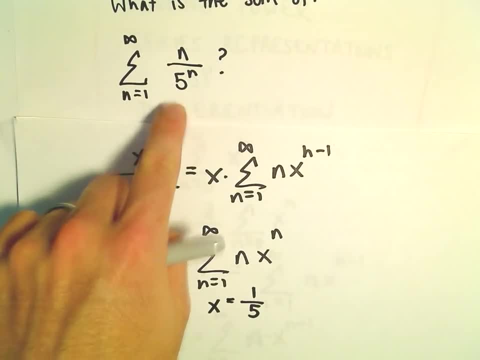 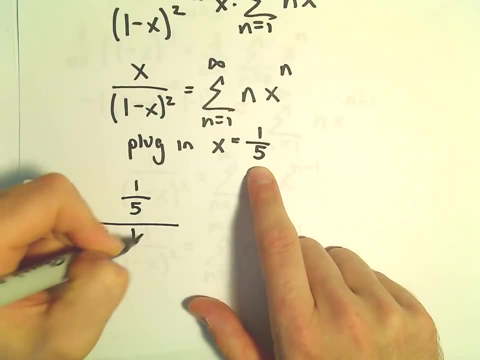 In this case, x equals 1 fifth. Okay, right, The 5 is in the denominator. If we plug in 1 fifth on the left, we have 1 fifth, 1 minus 1 fifth squared Well, on the right side we would have n equals 1.. 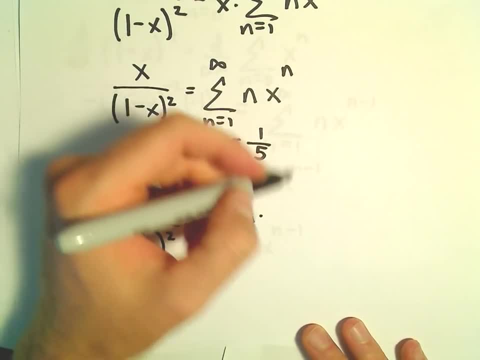 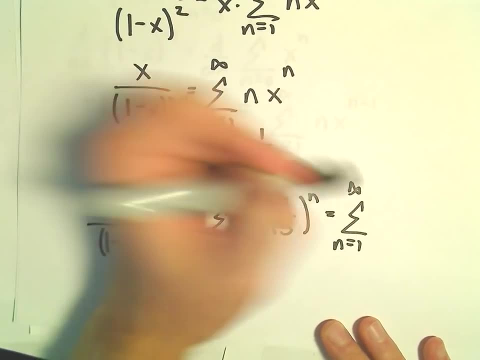 So n equals 1 to infinity of n times. well, let's see, we would have 1 over 5 raised to the n power. But again, we could actually rewrite this as n equals 1 to infinity of n over 5 to the n. 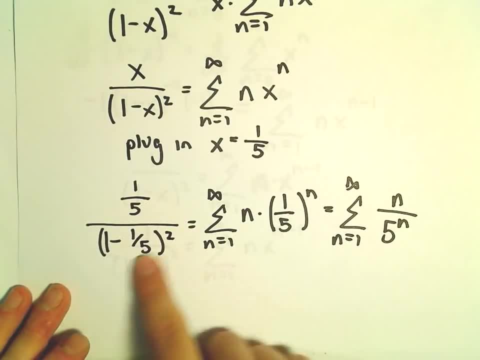 So, ha-ha, we finally figured out, you know, a way to compute it, because we've produced this formula on the left side. So, really, all we have to do is just compute the value of this, and now that'll give us our solution. 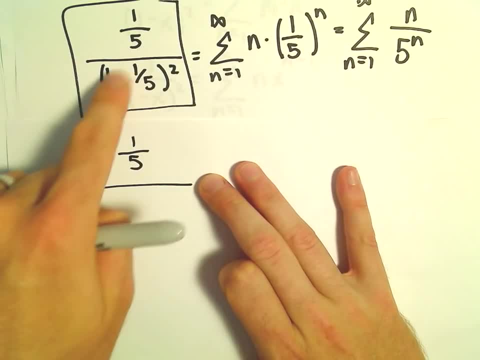 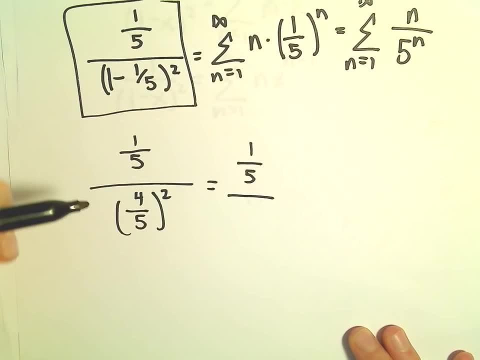 So let's see, We've got 1 fifth. So 1 minus 1 fifth is going to be 4 fifths Again. that's all going to be squared. So that's 1 fifth over 16 times 25.. 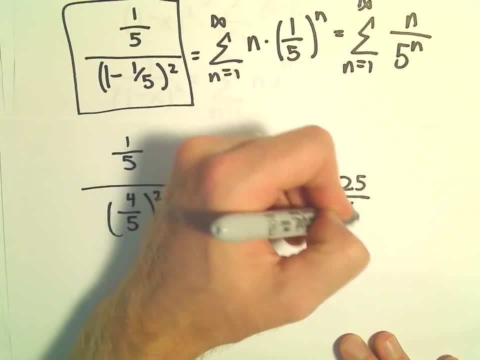 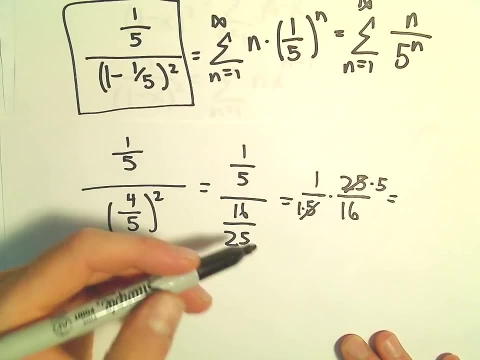 So that's going to be 1 fifth times 25 over 16.. Well, 5 goes into 5 once. 5 goes into 25 five times. So to me it looks like we're going to be left with the value 5 over 16.